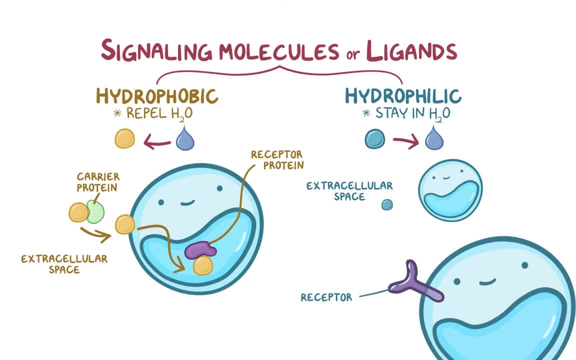 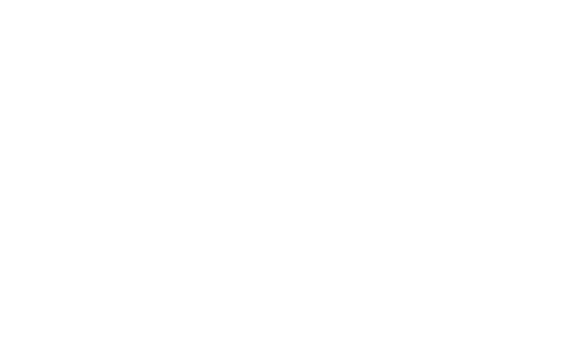 on the signal. hydrophilic molecules bind in receptors on the cell surface. These receptors are transmembrane proteins with an extracellular end that binds to the ligand and an intracellular end that triggers a signaling pathway inside the cell. We can think of the cell signaling pathway in three stages. the first stage is reception. 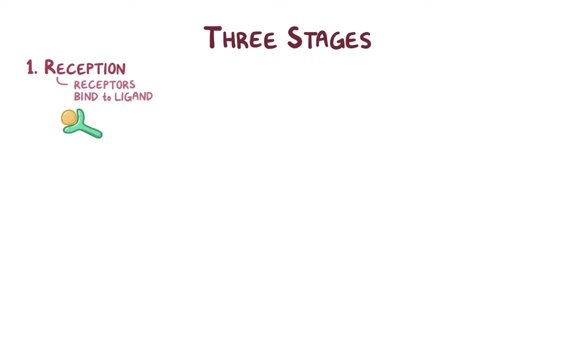 which is when the target cell's receptors bind to a ligand. Then there's transduction, which means that the receptor protein changes in some way and that activates intracellular molecules, the second messengers. The third stage is the cell's response to the signal. 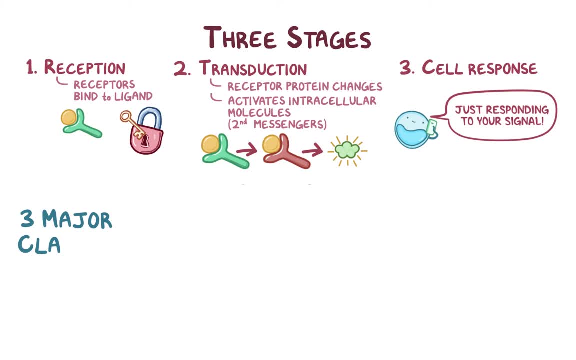 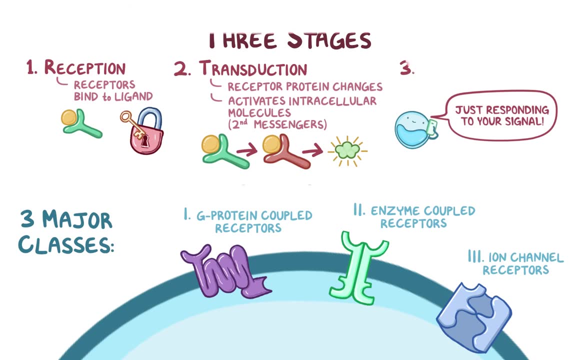 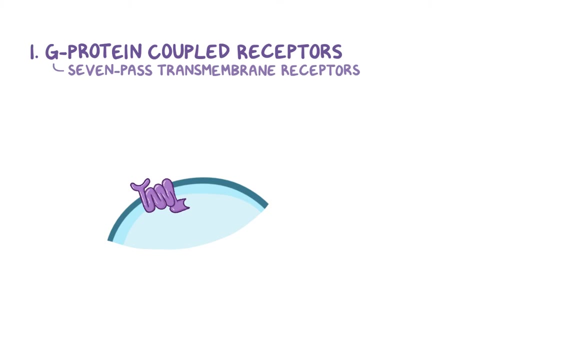 Zooming into these transmembrane receptors, there are three major classes: G-protein-coupled receptors, enzyme-coupled receptors and ion-channel receptors. G-protein-coupled receptors are seven-pass transmembrane receptors. These are like really long proteins. 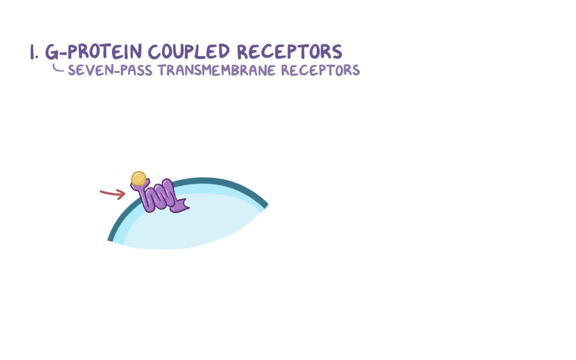 that have one end that sits outside the cell and binds the ligand. then the snake-like protein dips in and out of the cell membrane seven times and finally ends on the inside of the cell- The end of the G-protein-coupled receptor. 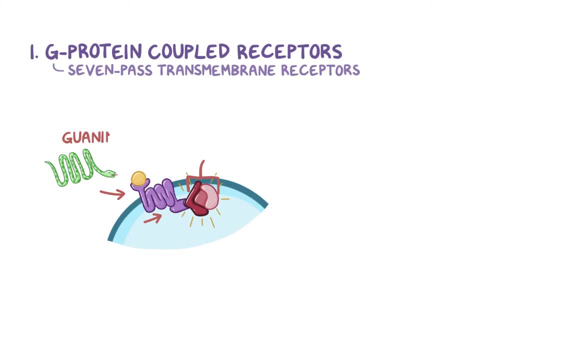 that's within the cell activates intracellular proteins called guanine, nucleotide binding proteins or G-proteins. G-proteins are made up of three subunits called alpha, beta and gamma, sort of like a flower with three petals. 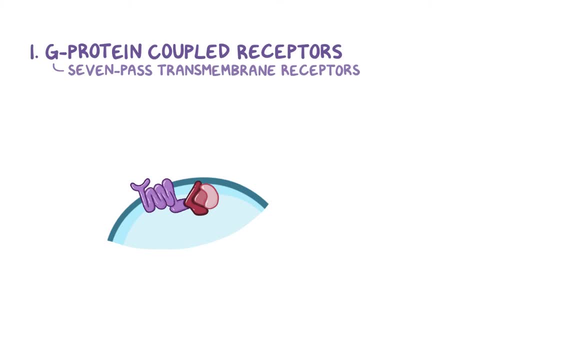 The alpha and the gamma subunits are anchored to the cell membrane and keep the G-protein right next to the receptor. G-proteins bind to guanosine diphosphate or GDP when they're inactive. When the alpha subunit is bound to GDP, 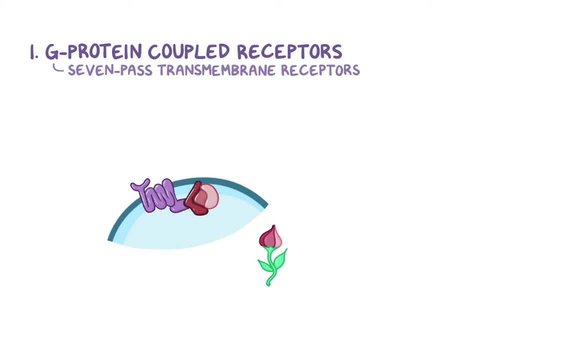 the three subunits stay together, so the flower is closed. But when the ligand binds, the G-protein-coupled receptor changes its shape and this allows the G-protein to release GDP and bind GTP, instead activating the protein. 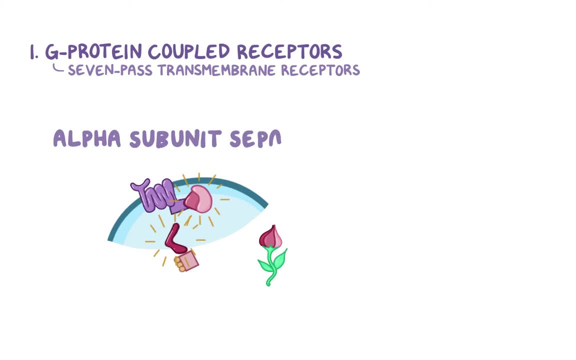 When the alpha subunit is bound to GTP, the alpha subunit separates from the beta and gamma subunits like one petal opening and separating from the others. When that happens, the alpha subunit is free to interact with other proteins. 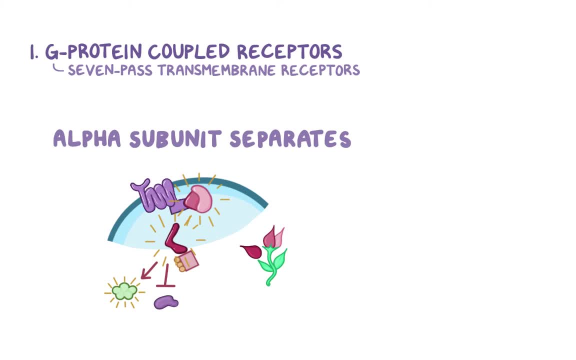 It stimulates some while inhibiting others. But to act on other proteins, the alpha subunit turns GTP into GDP and when that happens, the three subunits come together again, the flower closes and the G-protein is turned off. 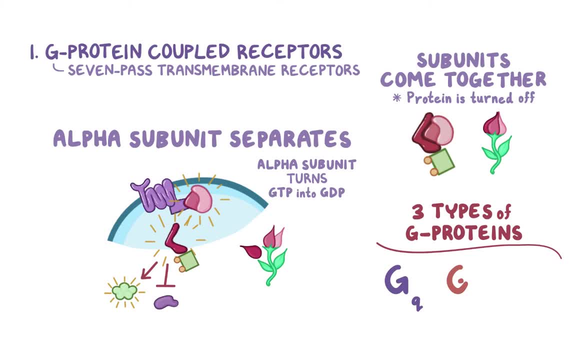 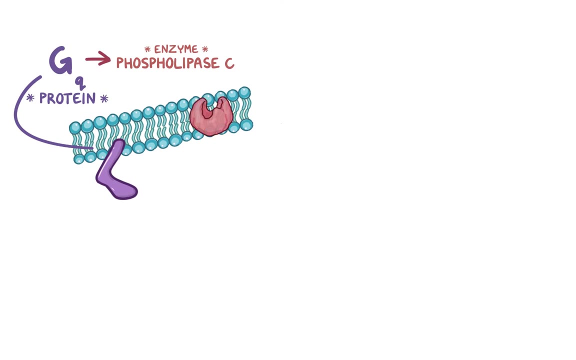 Overall, there are three types of G-proteins- GQ, GI and GS- and each one stimulates and inhibits a different set of enzymes and molecular pathways. The GQ protein activates the enzyme phospholipase C, which is found in the cell membrane. 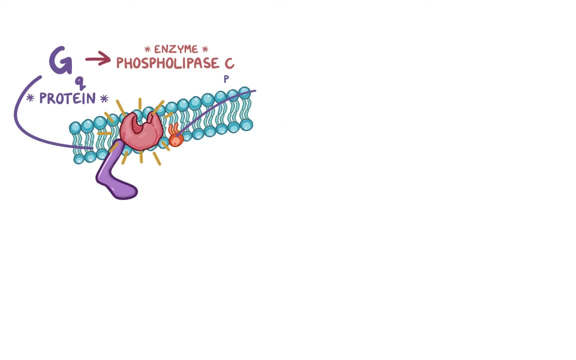 Phospholipase C then cleaves a phospholipid called phosphatidylinositol 4,5-bisphosphate into inositol trisphosphate and diacylglycerol. Inositol trisphosphate is soluble. 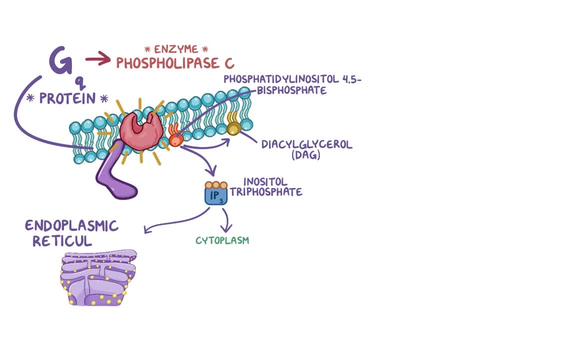 and diffuses freely through the cytoplasm and into the endoplasmic reticulum, where it opens up calcium channels. Since the calcium concentration is higher in the endoplasmic reticulum than in the cytoplasm, calcium flows out of the endoplasmic reticulum. 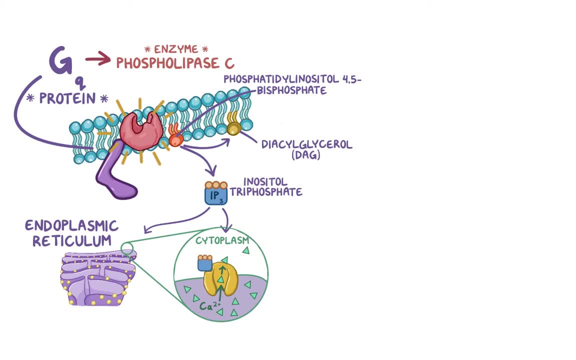 to the cytoplasm. The increased calcium concentration in the cytoplasm changes the electrical charge of the cell and can lead to depolarization. Meanwhile, diacylglycerol remains attached to the cell membrane and binds to the enzyme protein kinase C. 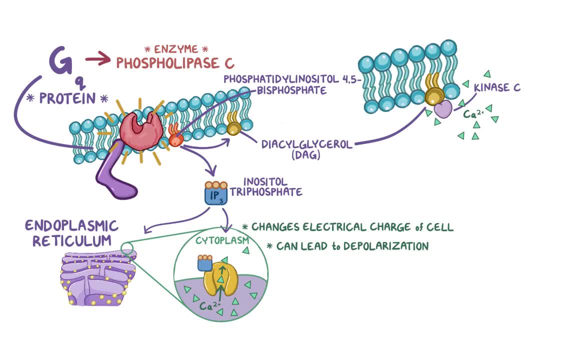 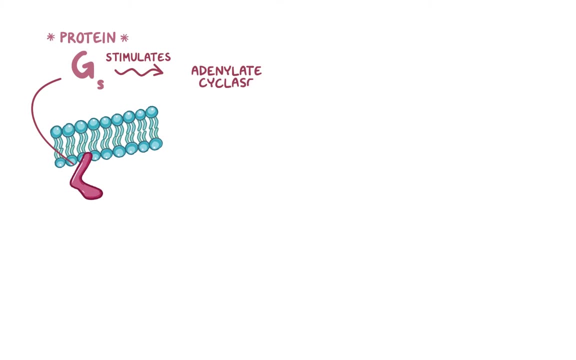 which also relies on calcium to fully activate. Once calcium levels in the cell go up, protein kinase C starts to activate proteins by adding phosphoryl groups to them. Next is protein GS, which stimulates the enzyme adenylate cyclase. Activated adenylate cyclase takes adenosine triphosphate. 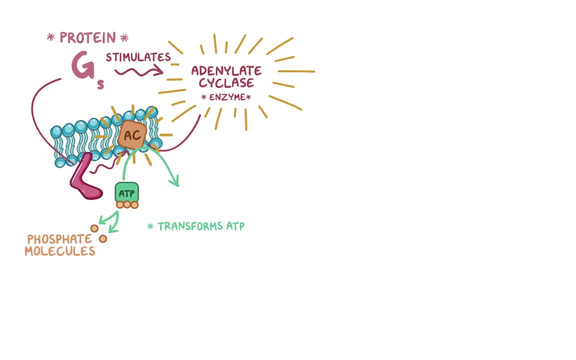 or ATP, and removes two phosphate molecules, transforming it into cyclic adenosine monophosphate or CAMP. CAMP moves throughout the cytoplasm and binds to the enzyme protein kinase A. Protein kinase A has two parts: a regulatory subunit and a catalytic subunit. 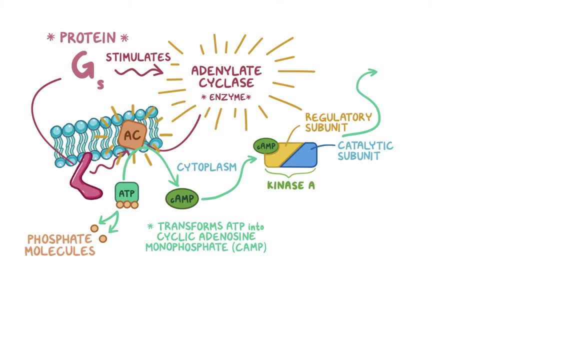 and CAMP specifically binds the regulatory subunit of protein kinase A. When CAMP binds, it makes the regulatory subunit dissociate from the catalytic subunit. It's kind of like pulling the pin out of a fire extinguisher allowing it in this case, it being the catalytic subunit. 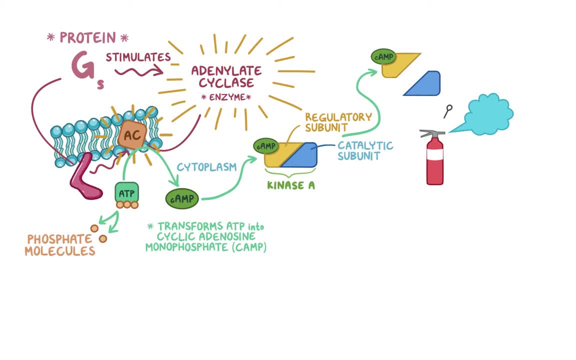 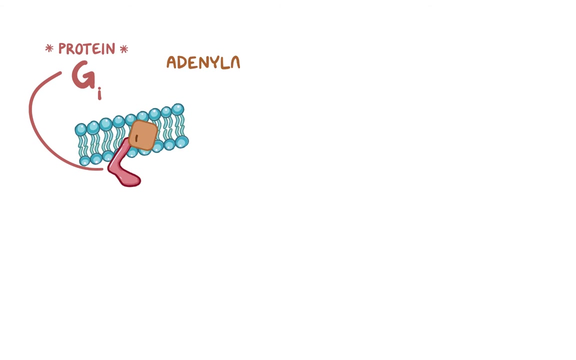 to do its job. So, after dissociating the catalytic subunit of protein, kinase A is free to phosphorylate target proteins that trigger a cellular response. Finally, there's the protein GI, which is also bound to adenylate cyclase. 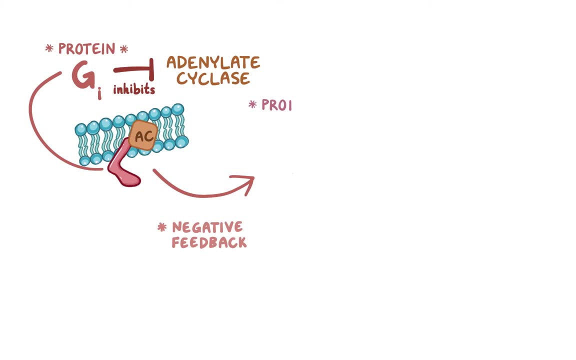 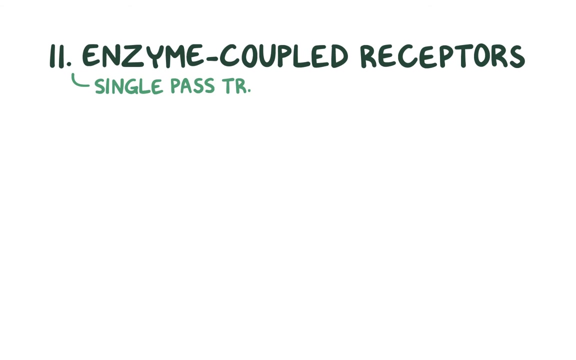 but in this case it inhibits it, causing negative feedback on protein GS. This is particularly important in helping to inactivate cells. Next are the enzyme-coupled receptors. They're usually single-pass transmembrane proteins, meaning that they have only one transmembrane. 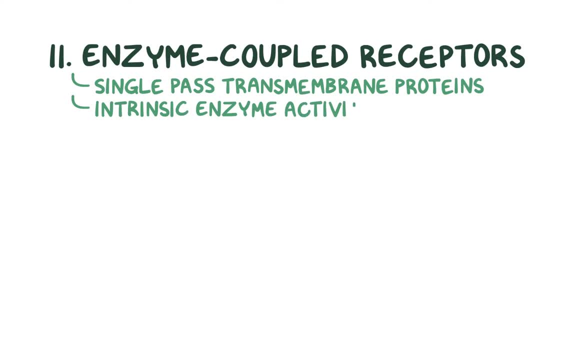 segment and their intracellular end has intrinsic enzyme activity. In other words, enzyme-coupled receptors have two parts. One domain is the receptor and the other domain is an enzyme. Each domain has a separate function, like on a Swiss Army knife that's composed. 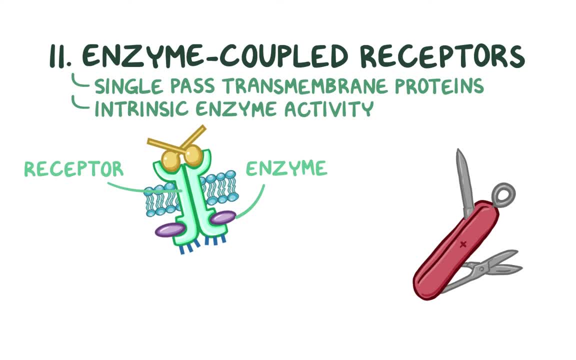 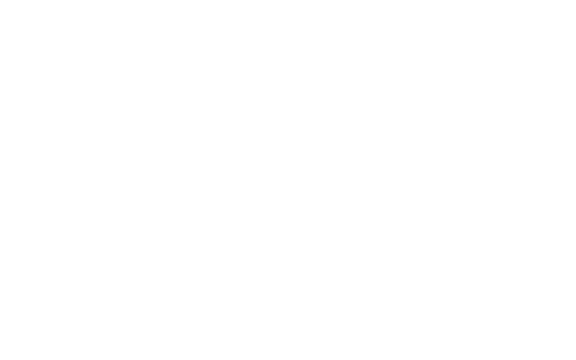 of both a knife and scissors. The enzymatic domain is usually a protein kinase that phosphorylates the receptor domain. Now there are three main types of enzyme-coupled receptors Based on the amino acid at which the receptors get phosphorylated. The first group are the receptor tyrosine kinases. 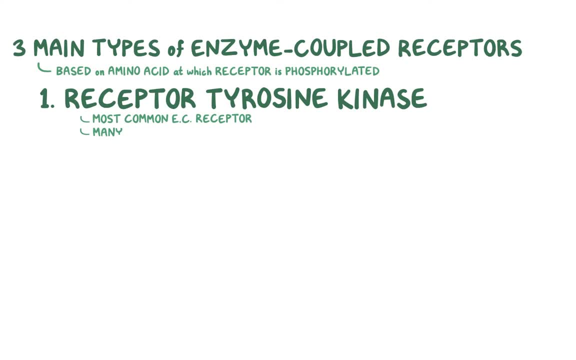 These are the most common enzyme-coupled receptors and there are many subfamilies. Receptor tyrosine kinase are generally molecules that can't phosphorylate their own tyrosine side chains. When a ligand binds, two receptor chains come together. 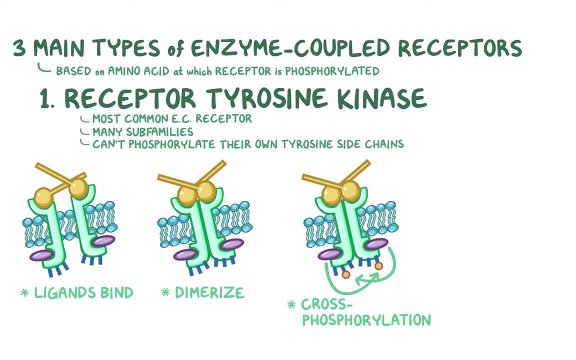 and dimerize and they cross-phosphorylate one another at multiple tyrosine residues. This triggers a conformational change that creates high-affinity binding sites for the second messengers, which can also be phosphorylated and activated, triggering the signaling pathway. 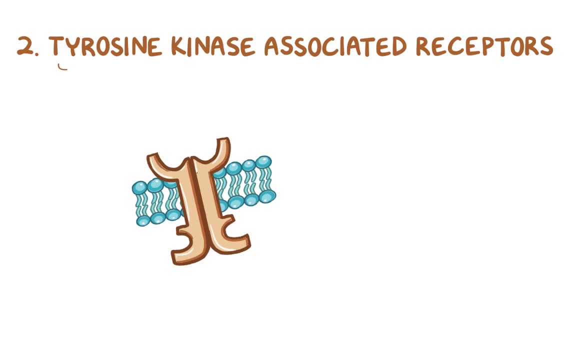 Next are the tyrosine kinase-associated receptors, which work in nearly the same way as receptor tyrosine kinases, And their name even sounds almost the same. The key difference is that they have no intrinsic enzyme activity. Instead, they're associated with cytoplasmic tyrosine kinases. 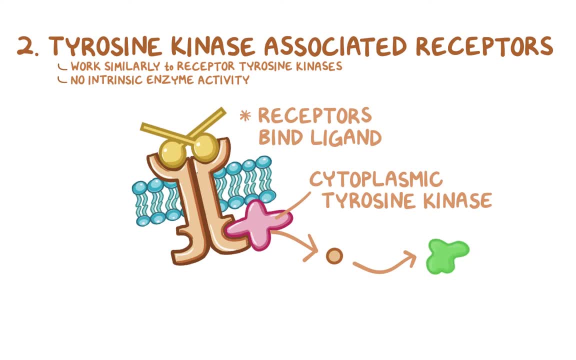 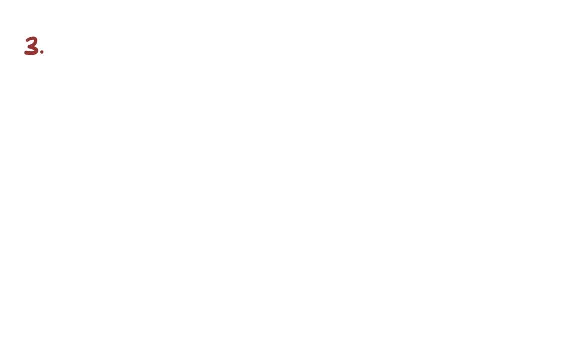 When the receptors bind their ligand, the cytoplasmic tyrosine kinases phosphorylate various target proteins to relay the signal. Finally, there are the receptor serine-threonine kinases and they have a serine-threonine kinase domain.